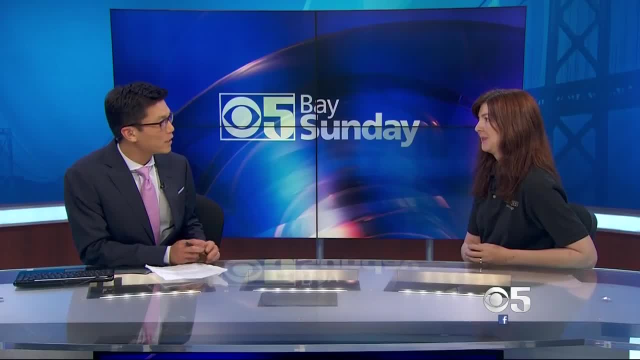 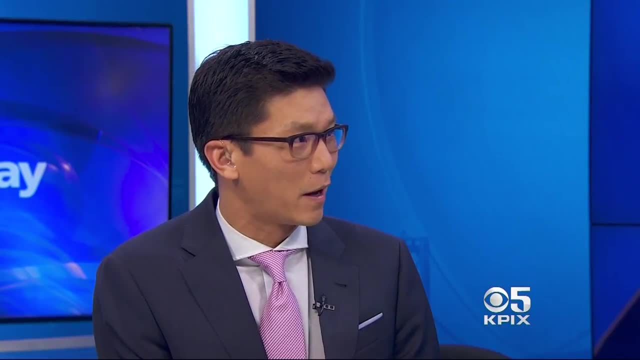 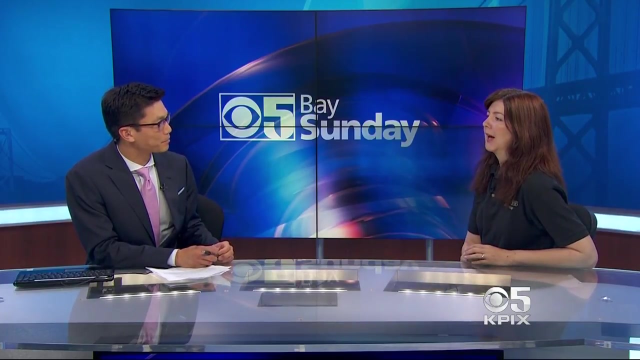 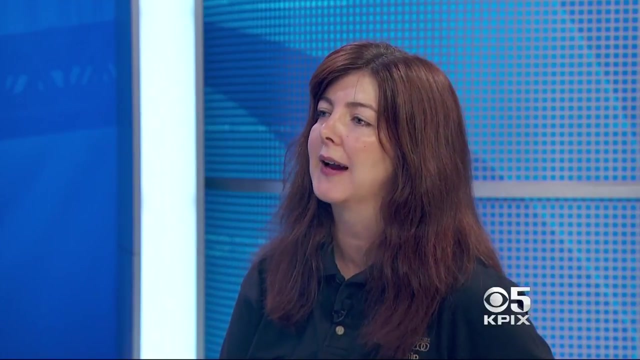 eight brand new animal exhibits. That sounds wonderful. And tell us about the gondola system that has been erected there at the zoo. A lot of people are excited about that in the Bay Area. I'm really excited about it And, I'll be honest, I ride this thing every chance I get Nice. So the new section of the zoo is up the hill from our current zoo, And so the way you access it is by an aerial gondola. It takes you up and over the hills. 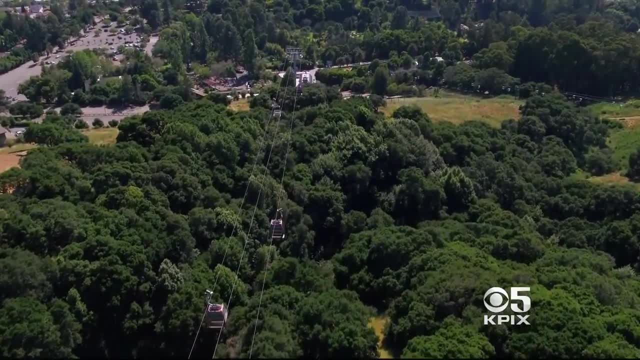 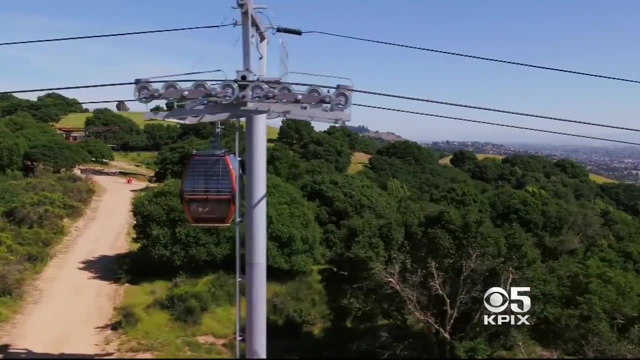 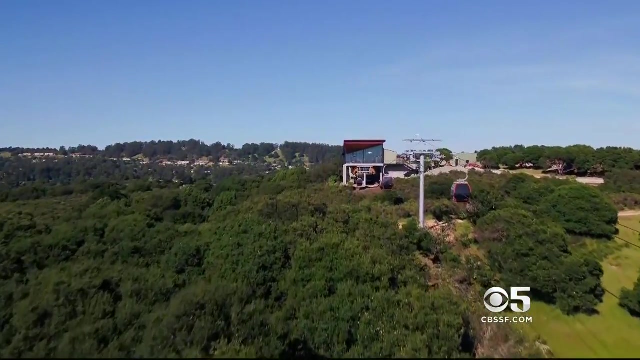 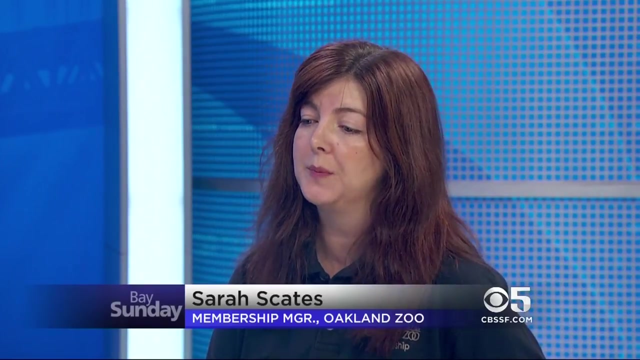 You get to look down on some of our current animals like the camels, and you can see the backside of elephants and lions, But the views of the bay are amazing. You can see the Bay Bridge, You can see the Golden Gate Bridge, You can see the skyline of San Francisco And then, right now, it just takes you up to our new restaurant called the Landing Cafe, And it's really, you know, what's open now is the first part of a new huge expansion for the zoo, So this year it's open to the public. 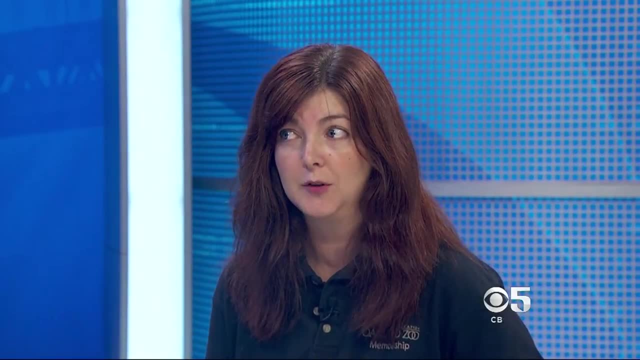 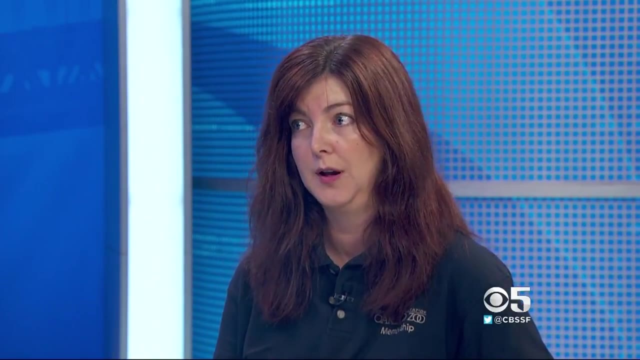 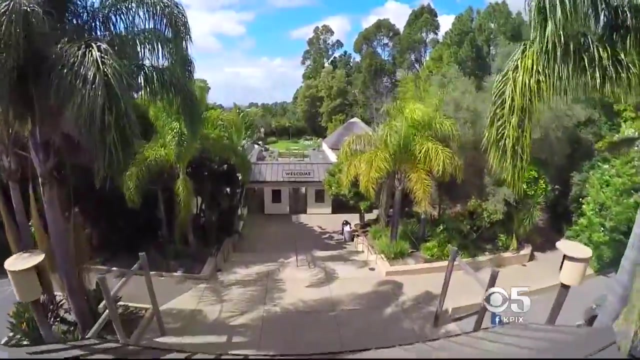 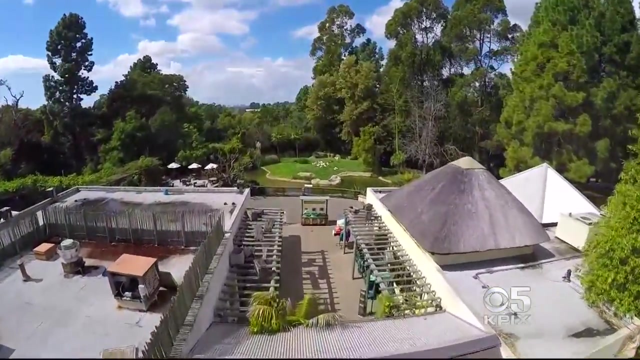 It's just the gondola and the new restaurant, And I want to make sure everybody knows that the gondola is included in your zoo admission or your membership, So it's not an extra fee. once you get to the zoo, The new restaurant has some delicious food, And then next year there will be eight new exhibits, a new playground and a new interactive science museum opening up, And I love this shot of the zoo as you enter the zoo right at the entrance. What is it about the zoo that makes it so special? 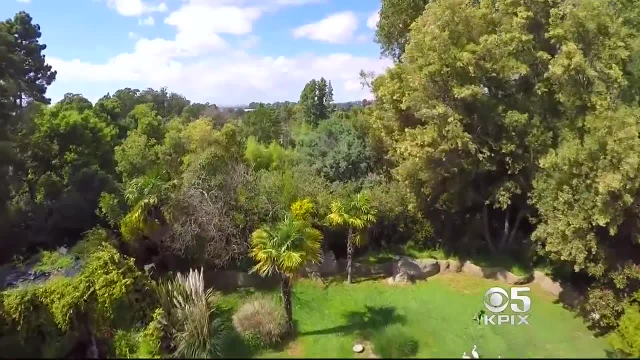 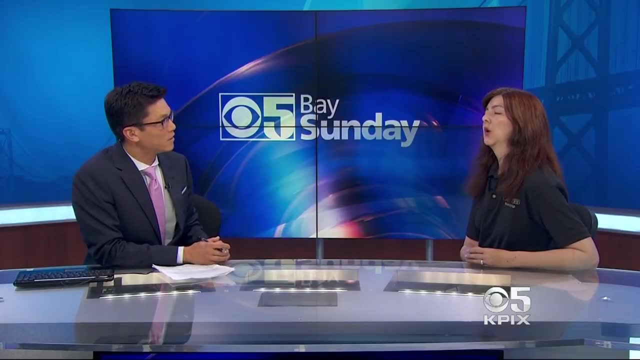 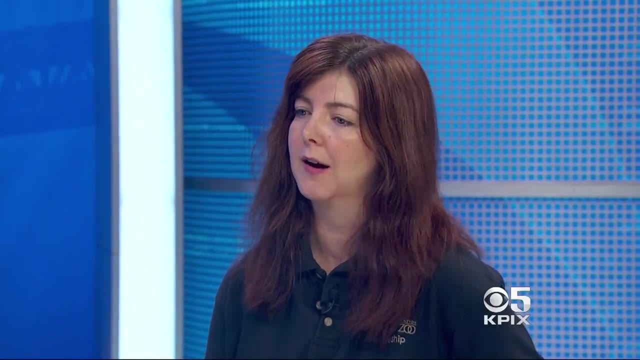 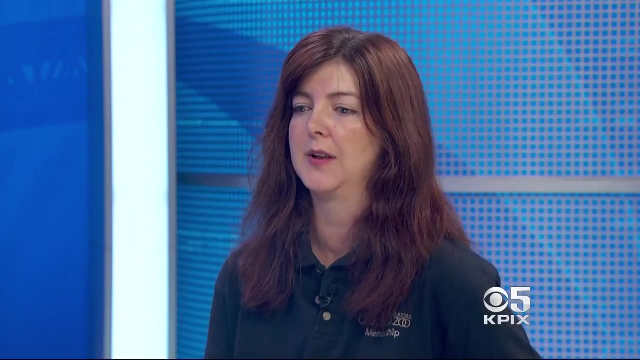 What makes this one special? I mean, I know there are so many zoos that you can visit here in the Bay Area and across the country, but it seems like you guys have a lot of new exhibits coming up and also some new animals that are appearing at the zoo. Yeah, So I think what makes the Oakland Zoo special is- and what gets mentioned a lot in our reviews by our visitors and members- is the animals are all in very naturalistic settings. We find that that's better for the animals and better for the people who come to visit, And so so that's very popular.